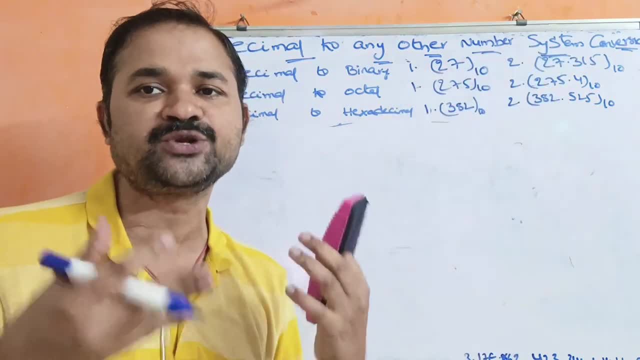 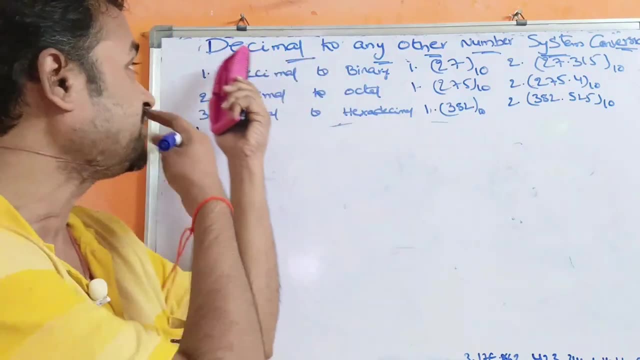 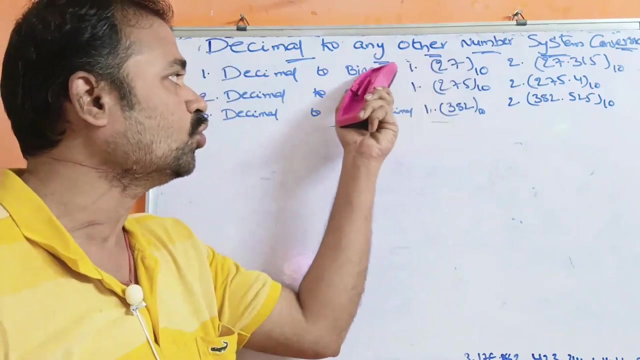 so we need to convert these two decimal numbers into the binary numbers. so d stands for decimal, d stands for division, assumes that d stands for division. so, simply, we need to perform the division operation. we need to perform division with 2. why? because the destination number system. 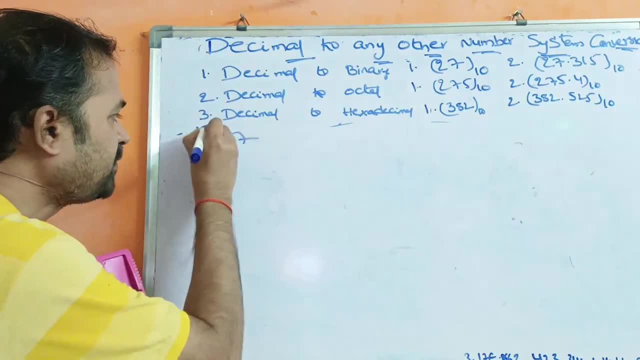 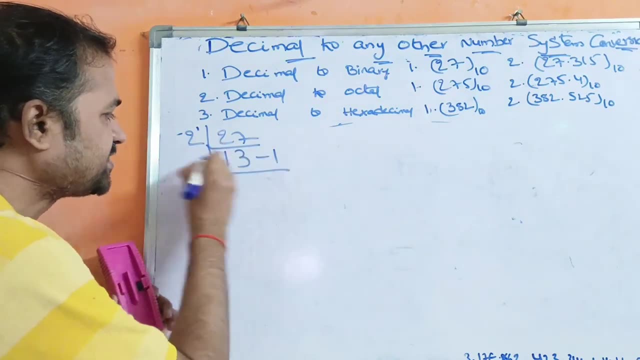 is binary, so 27, so simply perform the division operation. so two thirteens are 26, so 13 is the quotient, 1 is the remainder next. 2, 6 are twelfth. 6 is the quotient, 1 is the remainder, next two. 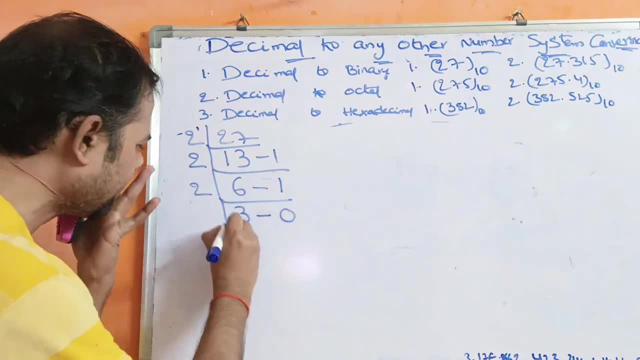 threes are 0, so 6 is the quotient. 1 is the remainder. next, 2 threes are 0, So 3 is the quotient. 0 is the remainder. Next to 2 ones are 2, 1 is the quotient. 1 is the remainder. 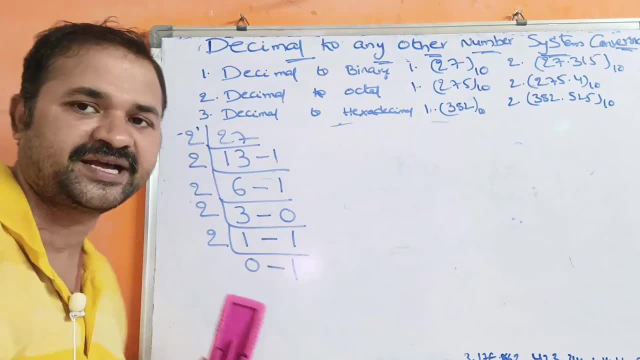 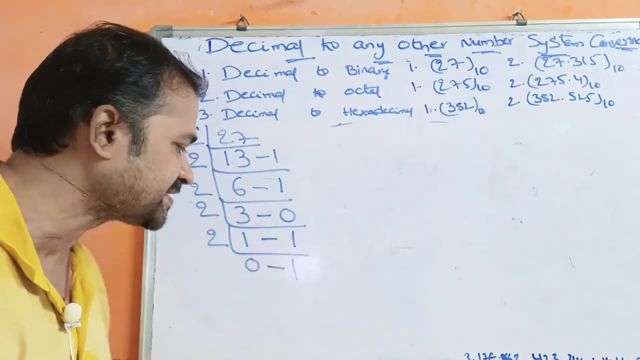 Next to 2 zeros are 0,. 0 is the quotient, 1 is the remainder. Now we can stop the process. Why? Because we got quotient as 0.. Here the resultant binary number is: we have to take from bottom to top. 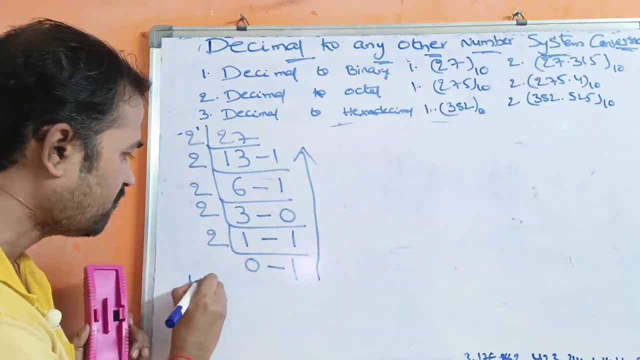 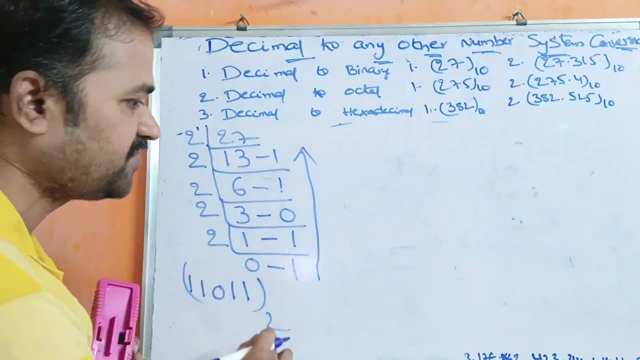 We have to take from bottom to top: So 1, 1, 0, 1, 1, base 2. So 1, 1, 0, 1, 1.. So 1, 1, 0, 1, 1.. 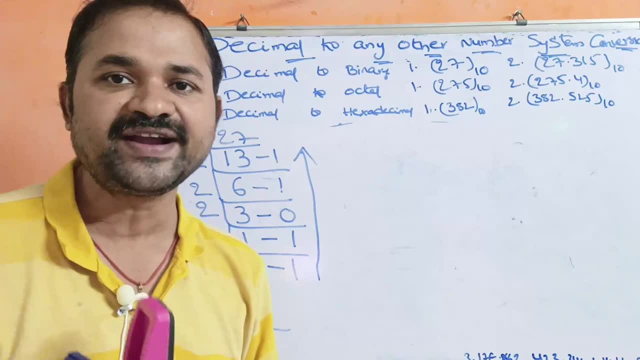 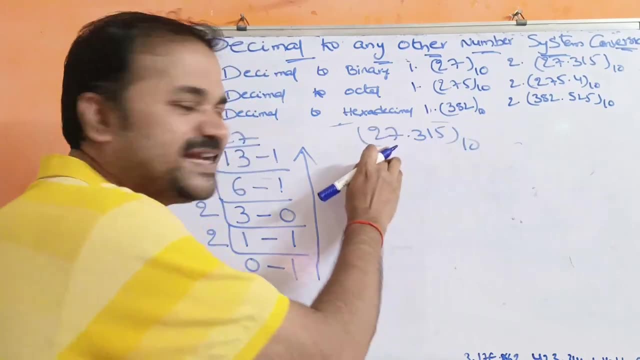 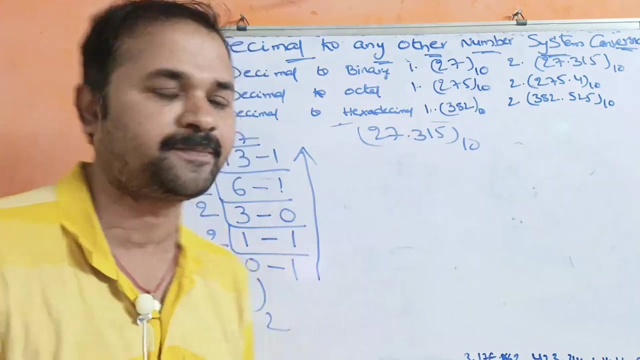 So this is the result. Next let us see the second example: 27.315.. 27.315 base 10.. So for integer part the binary number is already calculated. Now we have to calculate the binary number for the fractional part. 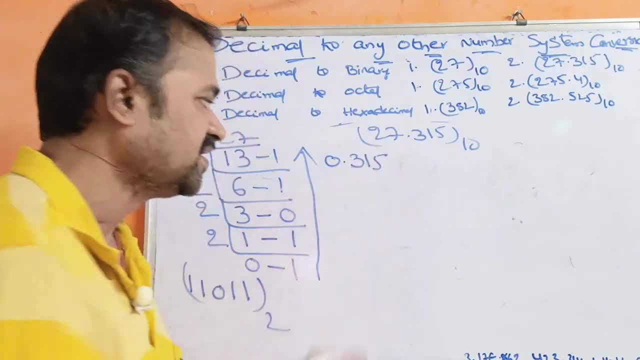 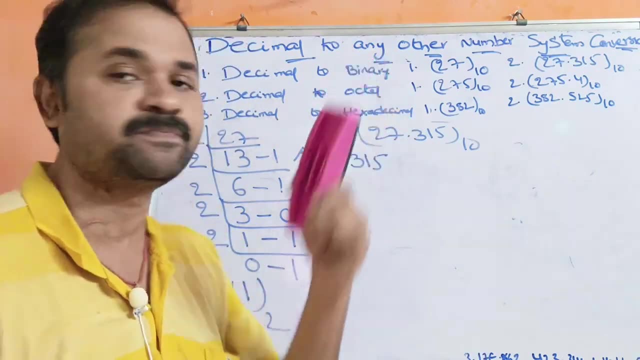 Here, what is the fractional part? 0.315.. For the fractional part, simply we need to perform the multiplication Multiplication operation Here. what is the destination number system? Binary number system. So simply we need to perform multiplication by 2.. 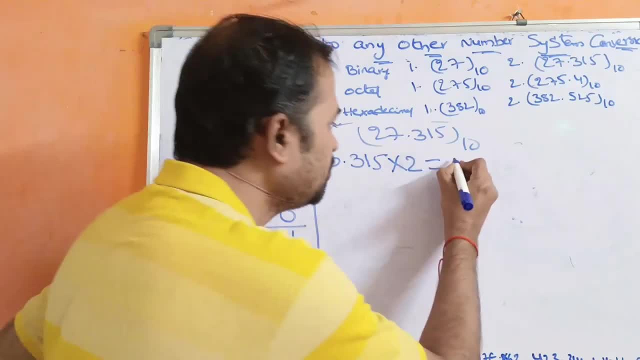 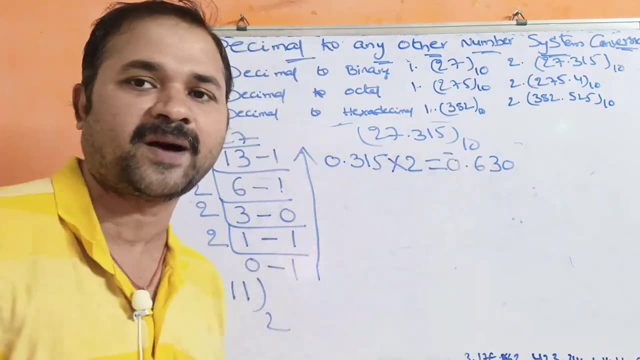 So 0.315 into 2 is equal to So 0.. So 2 3's are 6, 2 15's are 30. So here, what is the integer part? 0 is the integer part. 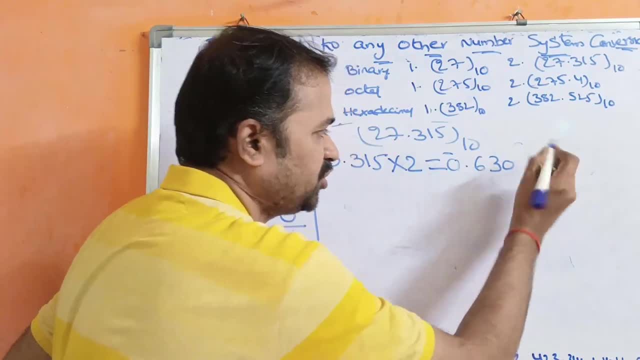 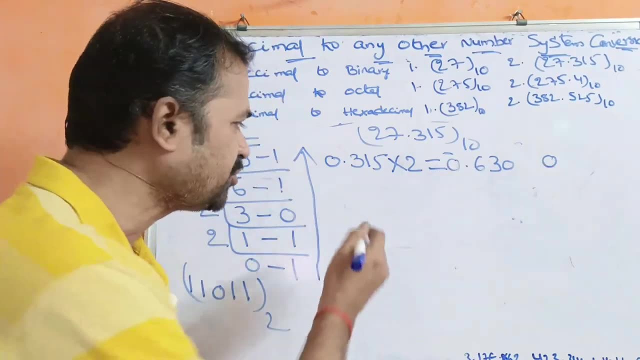 We have to extract the integer part and we need to write the 0.. After extracting the 0, there is no change in the integer part, So 0 minus 0. So we have to write it as 0.630.. 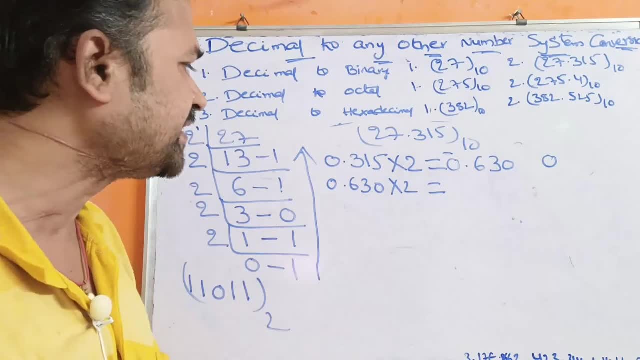 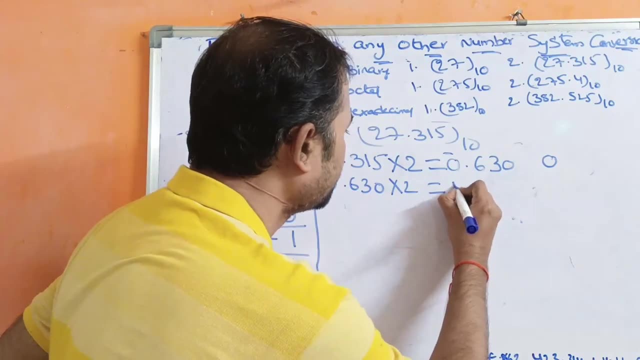 Again, we need to multiply this number by 2.. So 0.63 means 126.. So after one position we need to write that dot, So 1.260.. Here what is the integer part? 1 is the integer part. 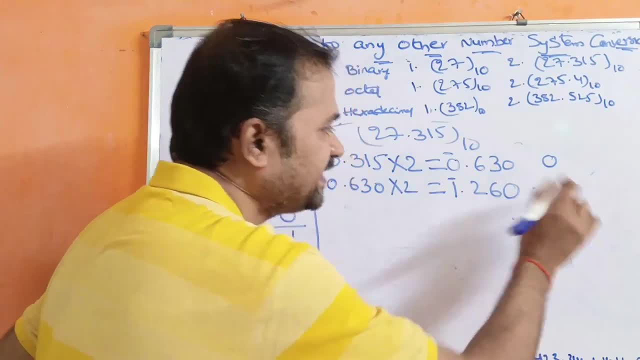 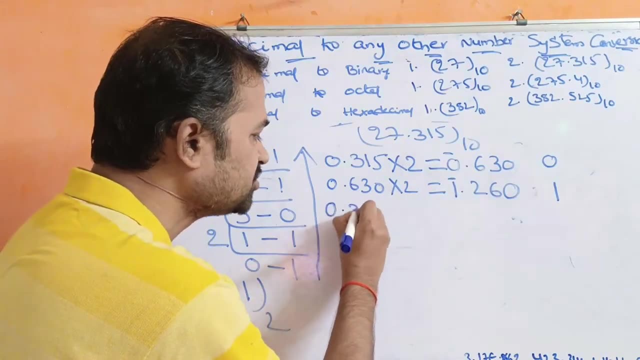 So we have to extract that integer part and we need to write that integer part here. So here 1 is extracted, So after that this will become 0.. So we need to write it as 0.26.. 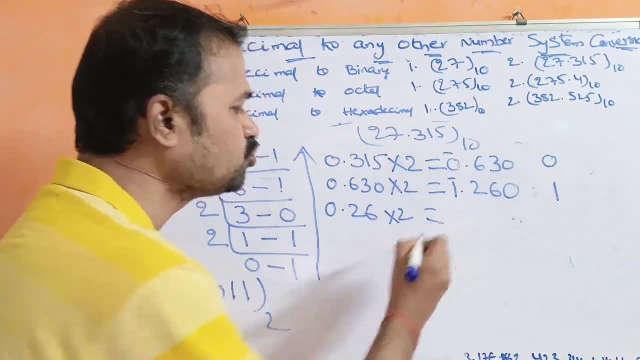 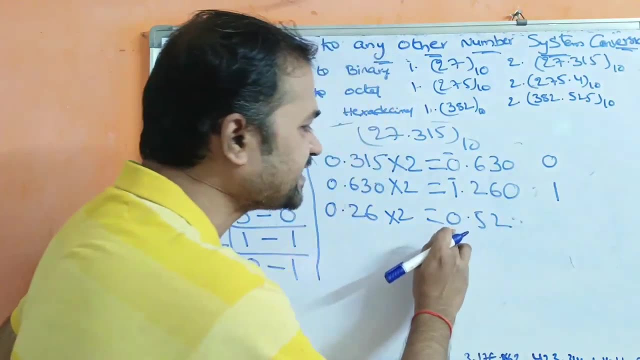 Why? Because 1 is extracted. So 0.26 into 2 means 0.26 into 2 means 52. So 0.52.. So let us extract the integer part and let us write here: So after extracting 0, the result won't change. 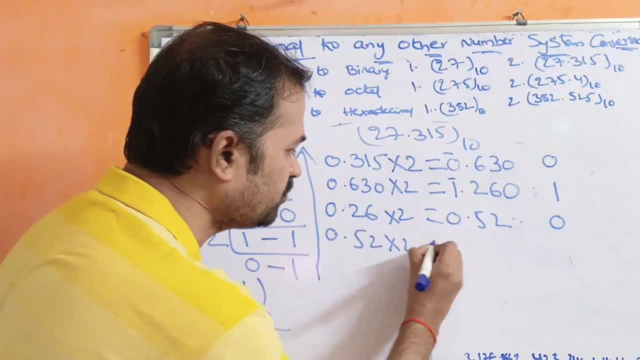 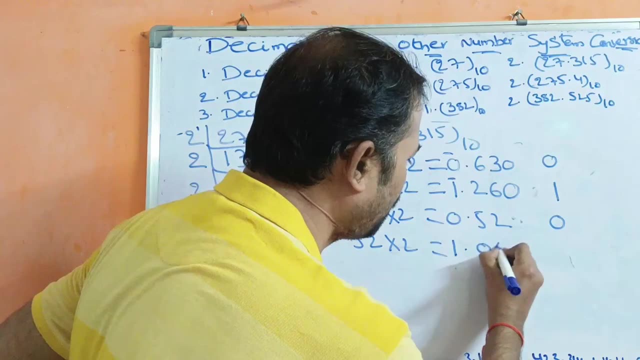 Integer part won't change. So 0.52 into 2 means. So 0.52 into 2 means 52, into 2 means 104.. So 1.05.. So here what is the integer part. 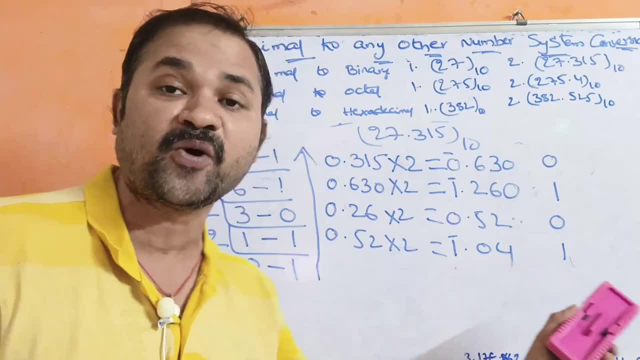 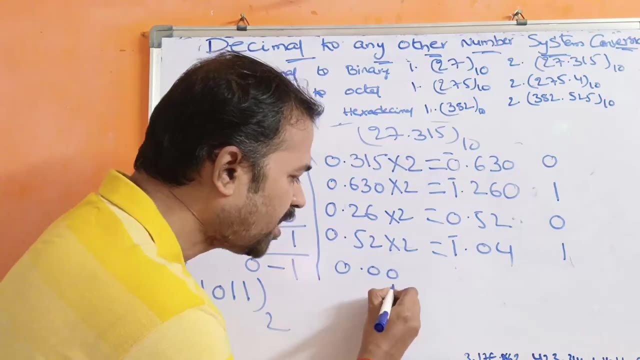 1 is the integer part. So after extracting 1, we got 0.04.. Here we need to repeat the procedure till we get 0.00, or 0.01,, 0.02, 0.03.. 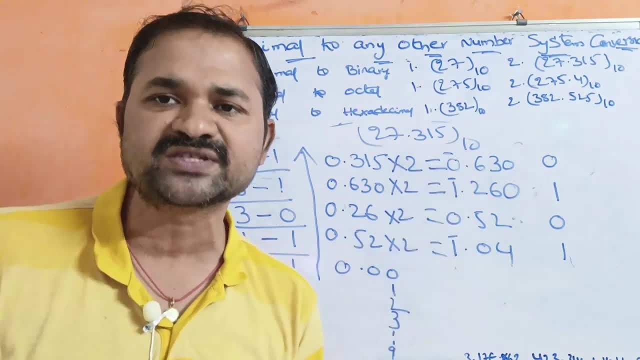 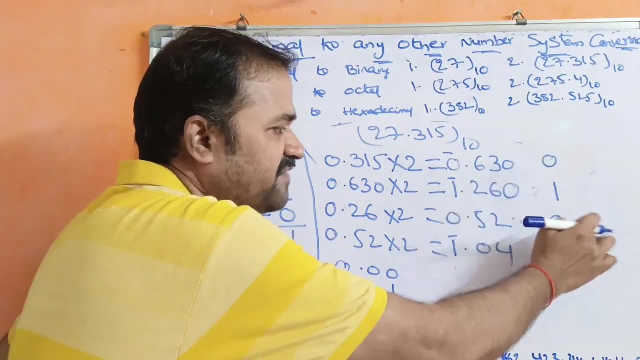 So on 0.09.. Or we have to repeat the process for 3 to 4 decimal points. So here we are having 3 decimal points, After that we are having 4 points. So now we can stop the process. 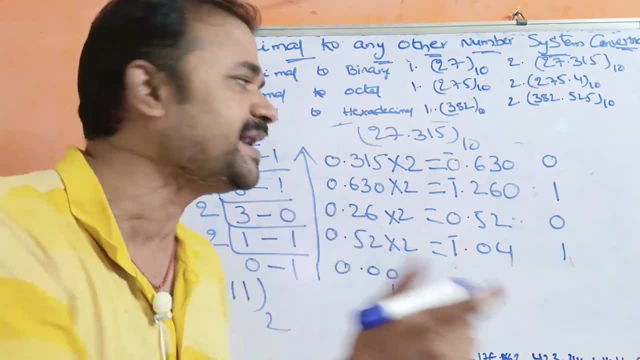 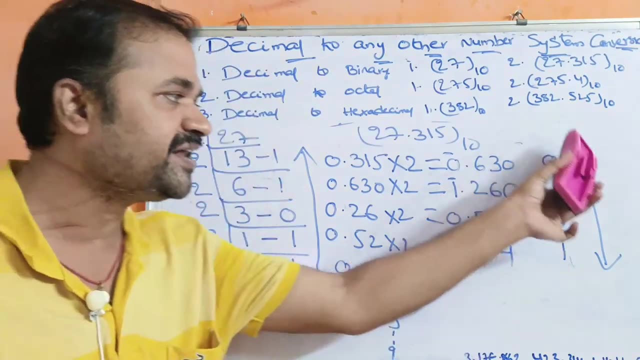 And for the fractional part we have to take the number from top to bottom. For integer part, we have to take the binding number from bottom to top, Whereas for the fractional part, for top to bottom- For 27,- what is the binding number? 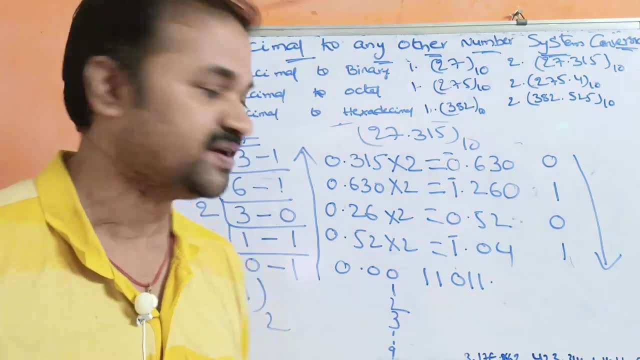 1, 1, 0, 1, 1.. 1, 1, 0, 1, 1.. Whereas for 0.315,, what is the result? 0, 1, 0, 1.. 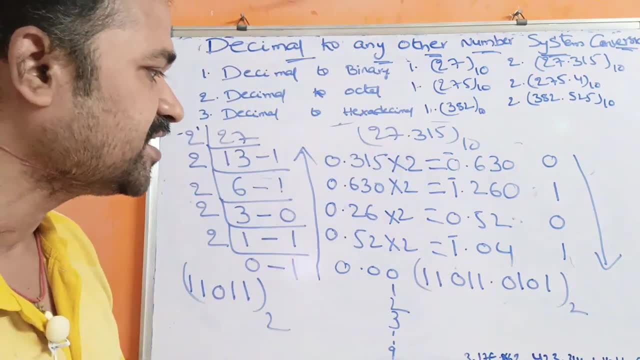 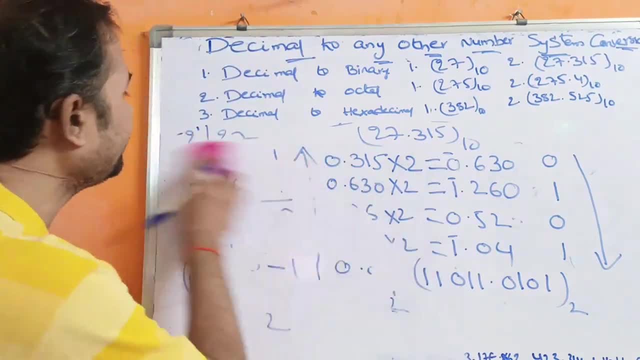 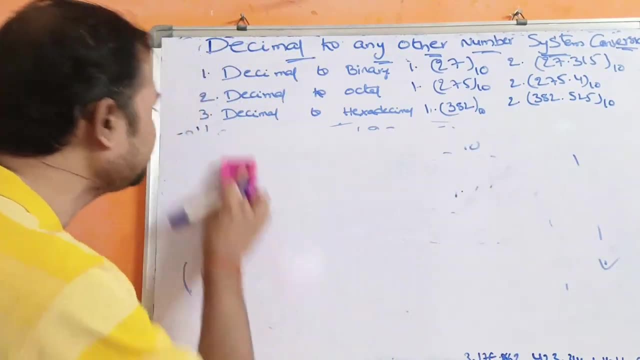 So decimal 2 binary conversion is over. Now let us see the second one. What is the second one? Decimal 2- octal conversion. So now we have to divide the decimal number by 8 till we get quotient as 0.. 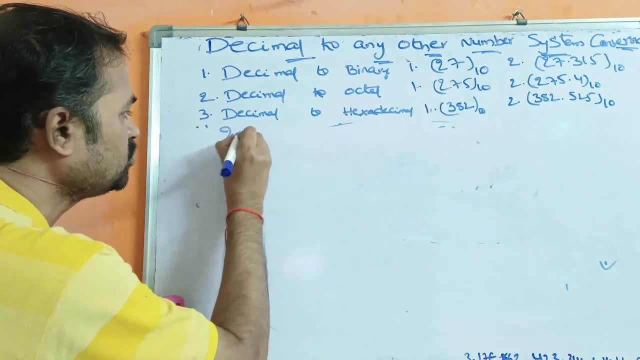 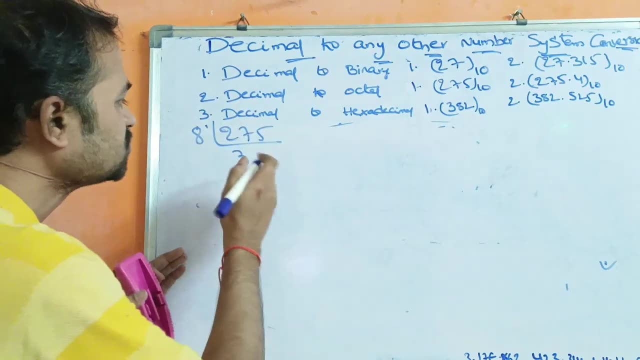 So what is the number? 275.. So 275.. So 8: 3s are 24.. 27 minus 24 means 3.. So 8: 4s are 32.. 32 minus 3.. 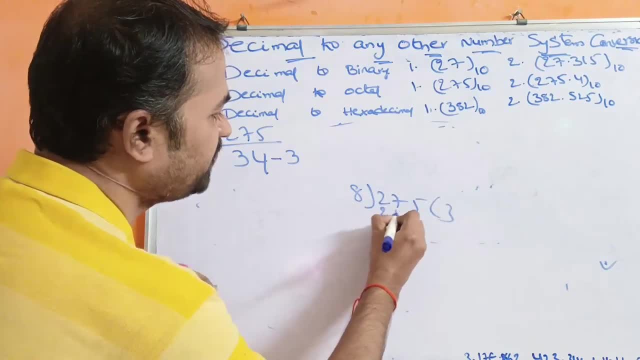 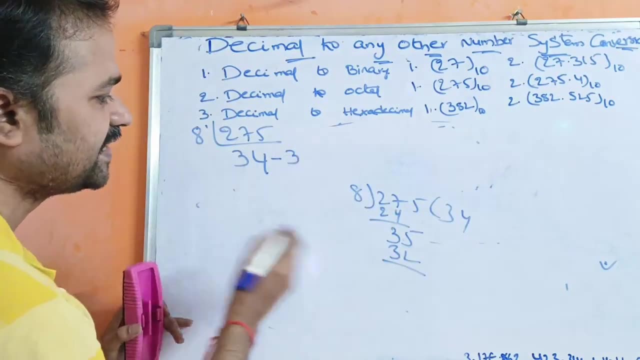 8, 275.. 8- 3s are 24.. 27 minus 24 means 3, 5.. 8- 4s are 32.. 34 is the quotient, 3 is the remainder. Next again, divide 34 by 8.. 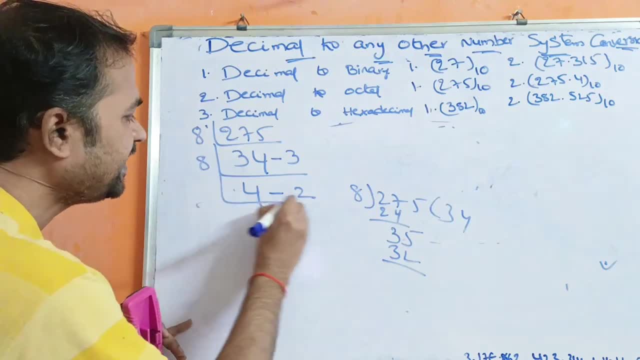 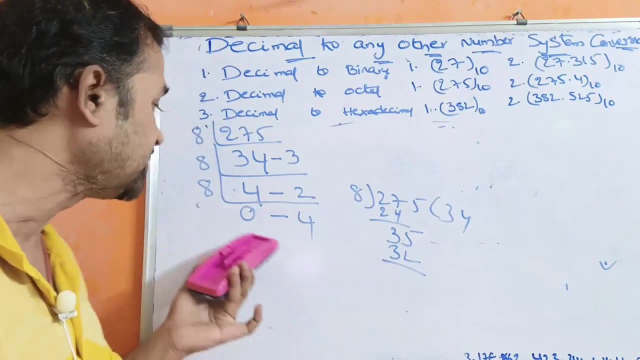 8: 4s are 32.. 2 is the remainder. Again, divide 4 by 8.. 8: 0s are 0, 4.. So now we can stop the process. Why? Because we got 0 as the quotient. 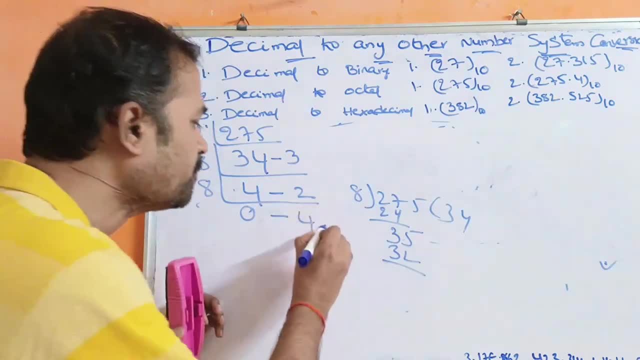 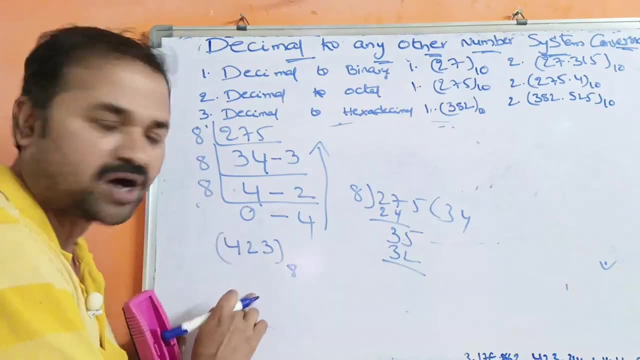 So for the integer part we have to write the number from bottom to top, So 423 base 8.. 423 base 8.. So this is the octal number for this decimal number. Octal means combinations of symbols from 0 to 7.. 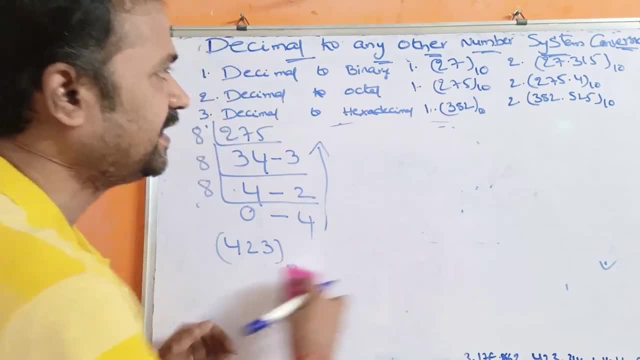 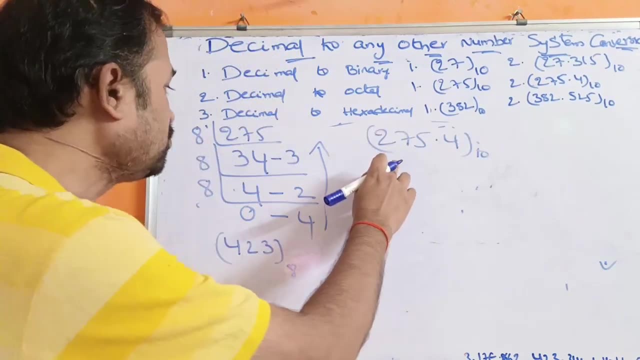 So 4 to 3 are from 0 to 7 only. Next let us solve the second problem: 275 dot 4 base 10.. For 275.. Already it is calculated. Octal number is already calculated. 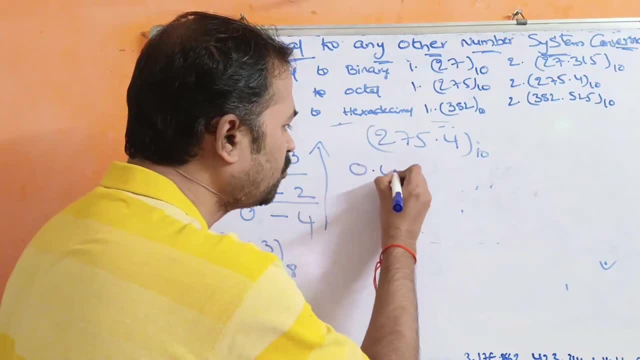 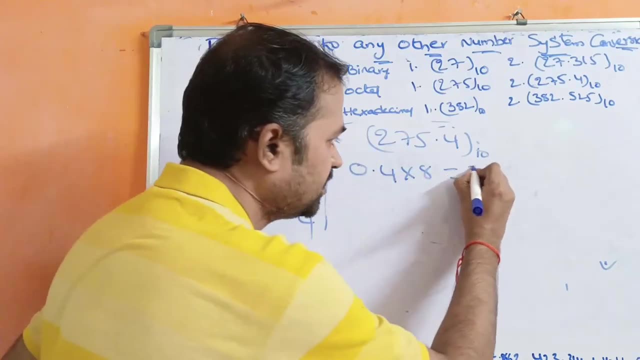 Now we have to calculate for dot 4.. So 0.4 into 8 is equal to What is the result? 8 4s are 32.. But after one position we need to write the dot, So 3.2 is the result. 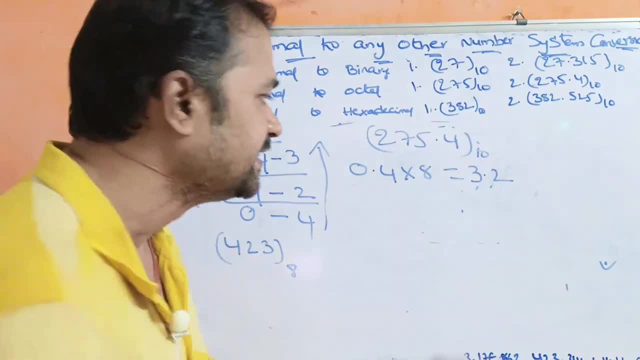 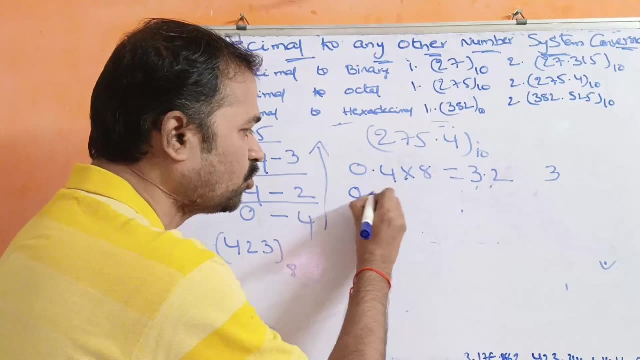 3.2 is the result In 3.2, what is the integer part? 3 is the integer part, So extract that integer part and write here. So after extracting 3, integer part will become 0.. 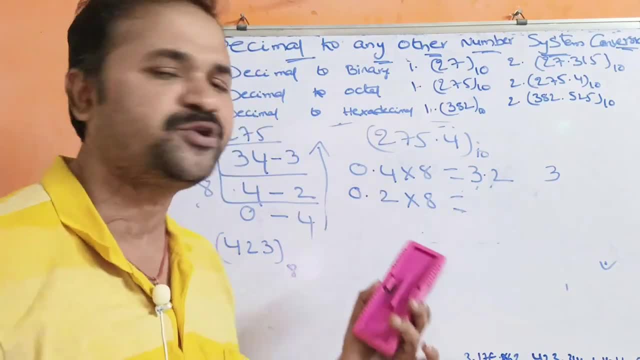 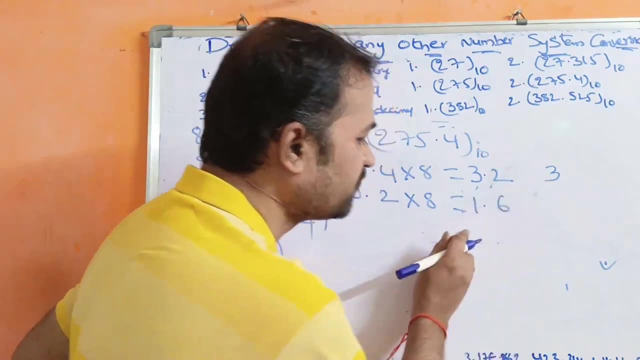 So 0.2 into 8.. So 0.2.. So 0.2 into 8 means 16.. So after one position we have to write the dot So 1.6.. So in 1.6, what is the integer part? 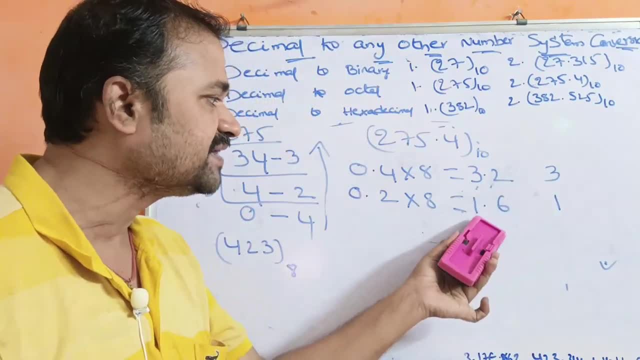 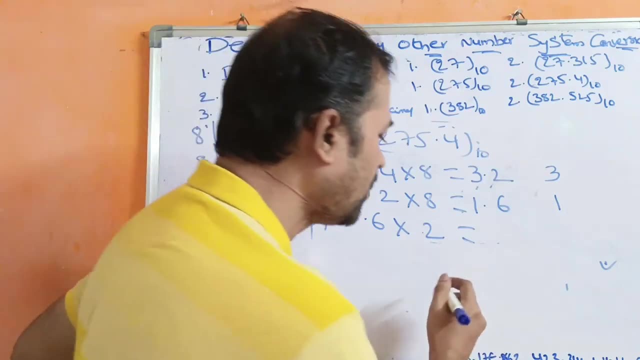 1 is the integer part. So after extracting 1, the integer part will become 0.. So 0.6 into 2 means 6, into 2 means 1.2.. Okay, 1.2.. 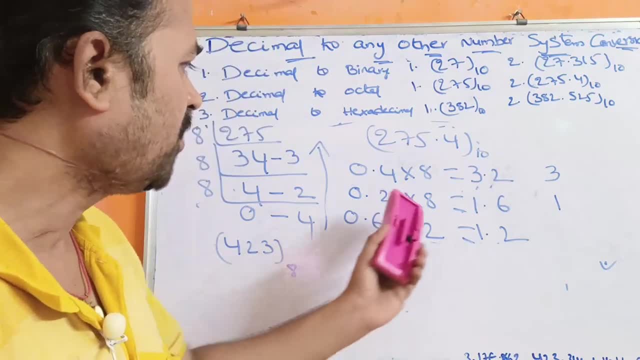 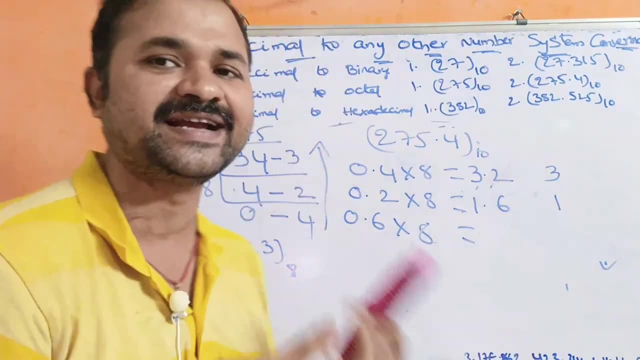 1.2.. So 0.2 into. I am sorry Here, what is the number? 8 is the number 8, is the number? So 0.6 into 8 means 8.6 or 48.. 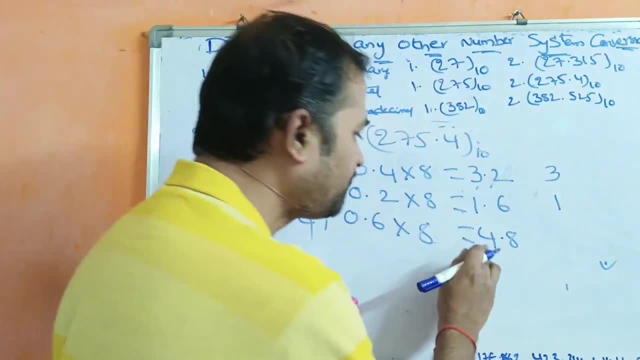 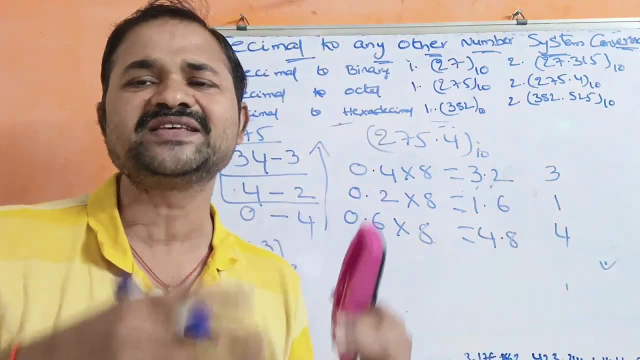 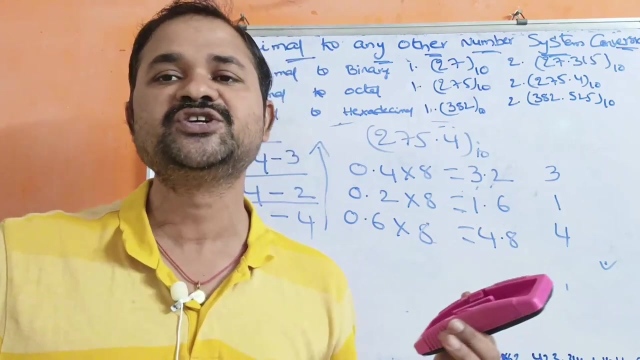 So after one position we need to write the dot, So 4.8.. So after extracting the integer part, So let us write here: So after that we will get 0.8.. So likewise, if we do the procedure, then there is no possibility to get 0.01, 0.02, 0.00.. 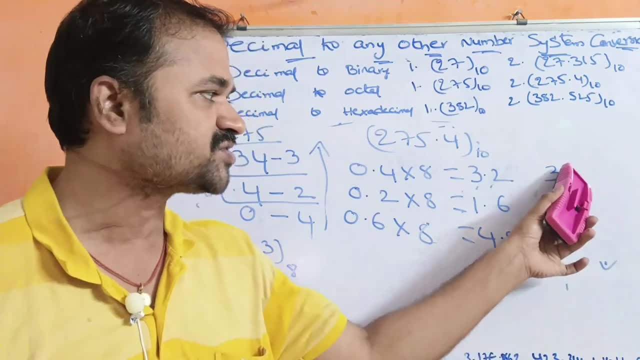 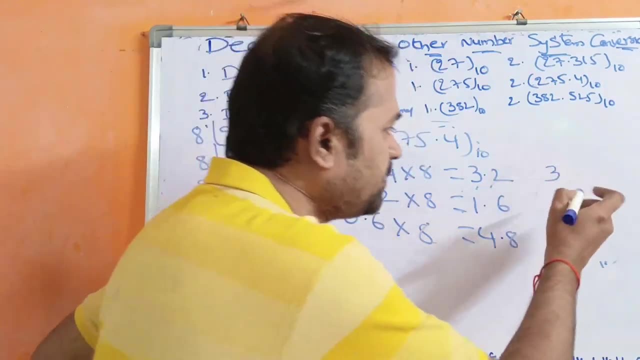 So that's why we need to stop the process now. Why? Because after the dot we have calculated for 3 points, 3 decimal points. So for the fractional part we need to write the number from top to bottom. 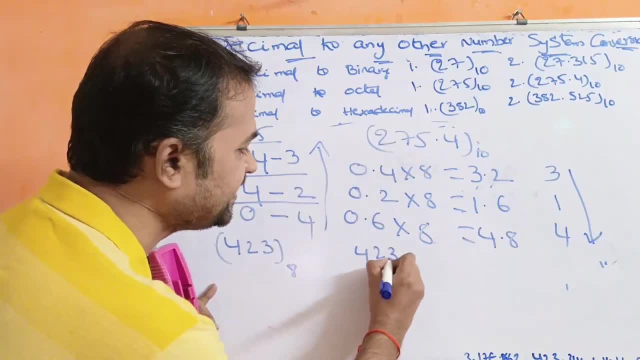 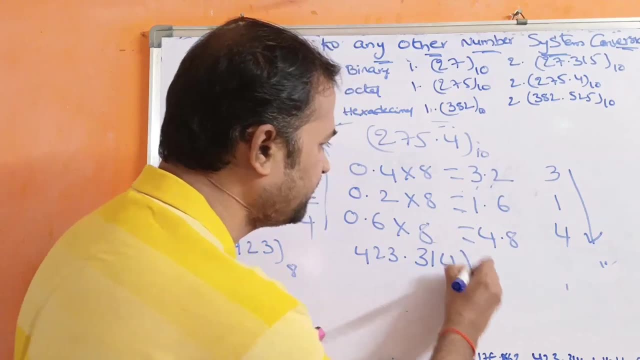 So for 275,. what is the octal number? 423 is the octal number So 423 dot For 0.4,. what is the octal number? 314 is the octal number Base? what is the base value? 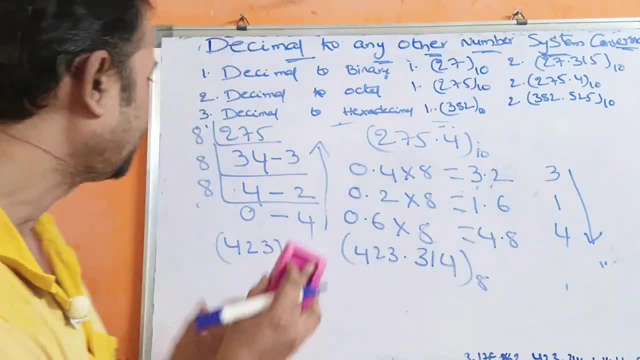 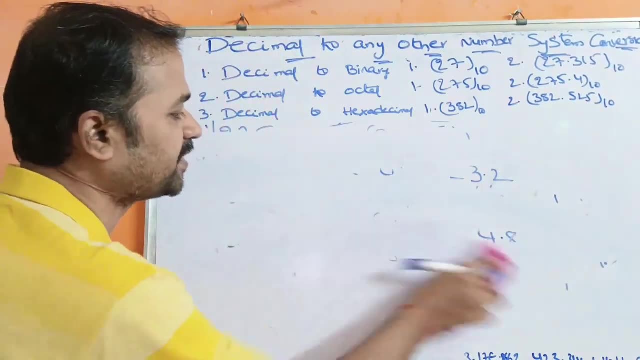 8 is the base value, So this is the solution. Okay, So with this decimal, 2, octal is also over. Now we need to convert decimal To hexadecimal number, So we need to divide that number by 16.. 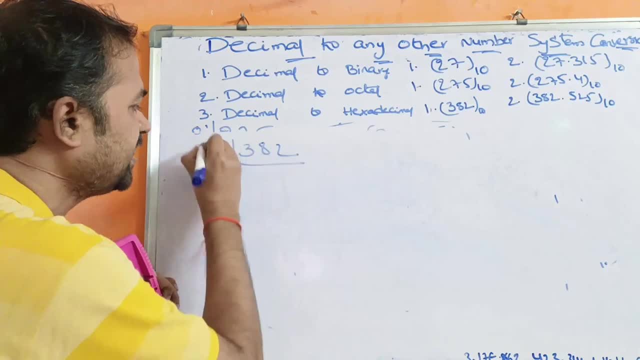 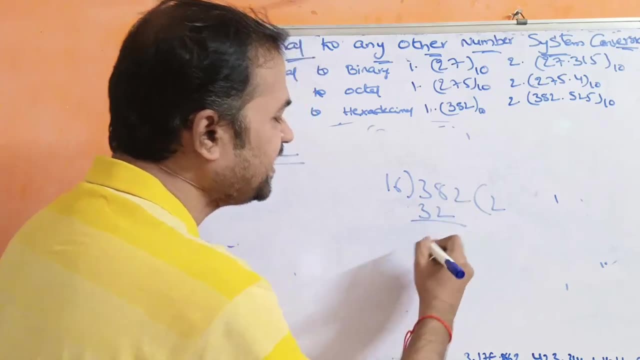 So here what is the number? 382.. 382.. So 16, 382.. So 16 2s are 32.. 32.. 38 minus 32 means 6.. Next, 16 3s are 48.. 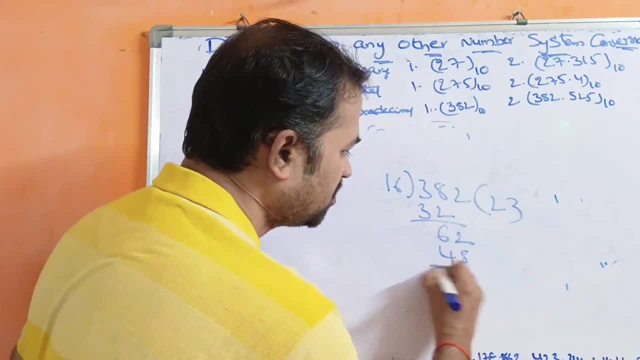 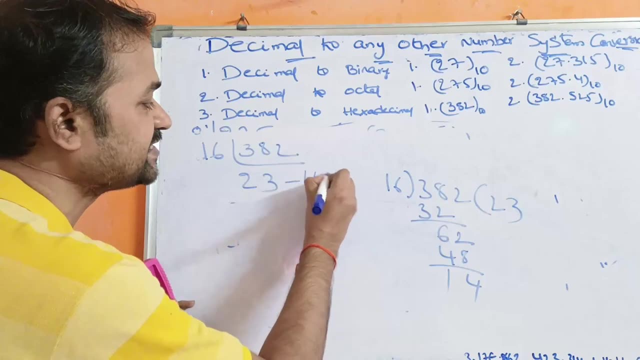 16 4s are 64.. 16: 3s are 48.. 12 minus 8 means 4.. 5 minus 4 means 1.. So what is the quotient 23? is the quotient 14? is the remainder. 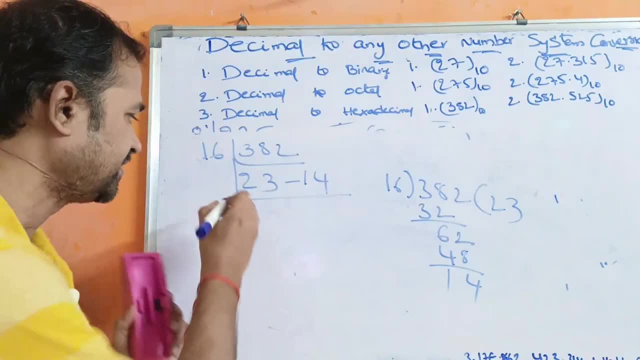 Next 16 1s are 16.. 16 2s are 13.. So 16 1s are 16.. So 23 minus 16 means 7.. Next 16 0s are 0.. 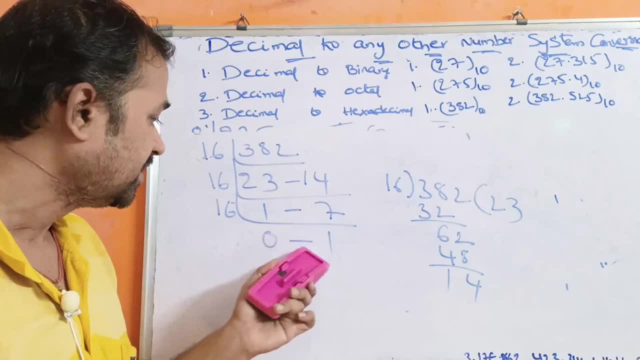 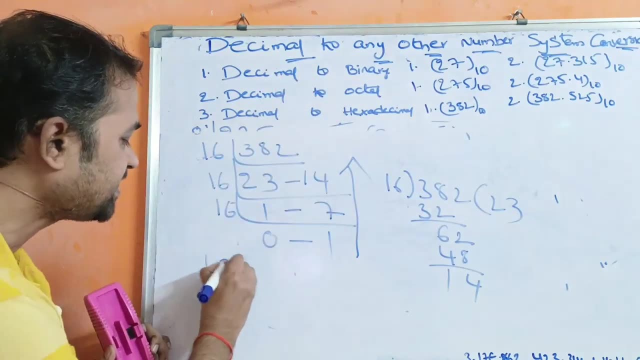 So 1 is the remainder. Okay, 1 is the remainder. So now for the integer part. we have to take from top, bottom to top, So 1,, 7,, 14.. So in hexadecimal system 10 means A. 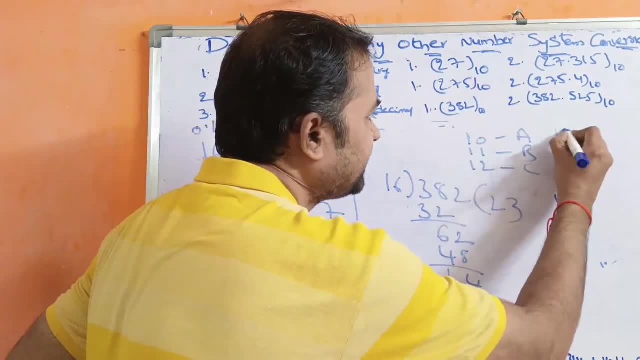 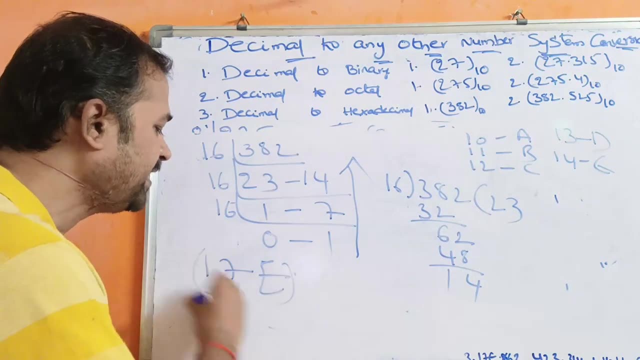 11 means B, 12 means C, 13 means D, So 14 means E, So this 14 means E, So 1, 7, E, base 16.. So this is the solution for this problem. 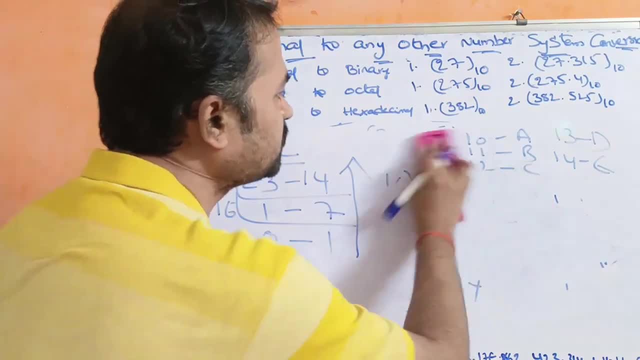 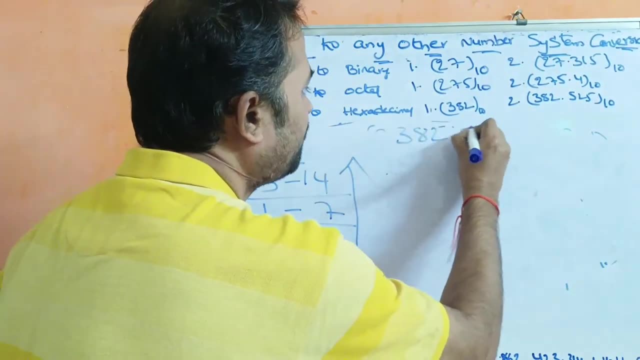 1,, 7, E. So now we have to solve the second problem. What is the second problem? 382, dot 382, dot 525, base 16.. For 382, already hexadecimal number is calculated. 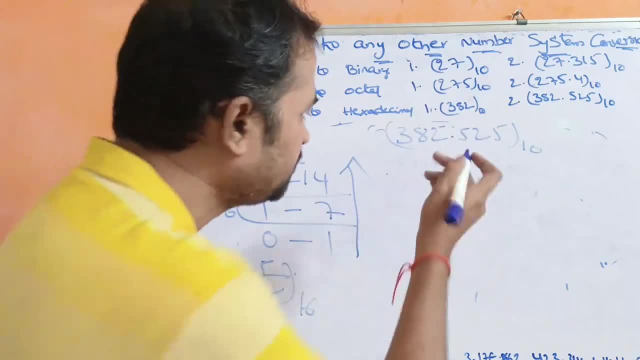 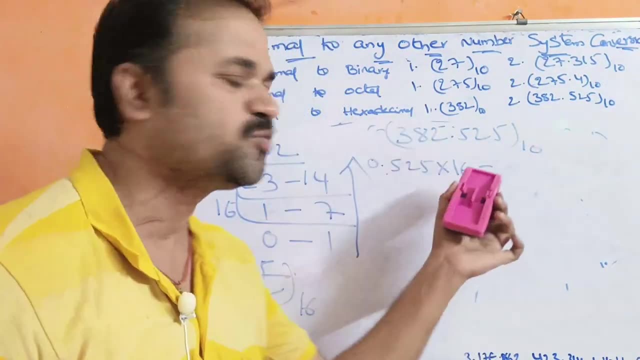 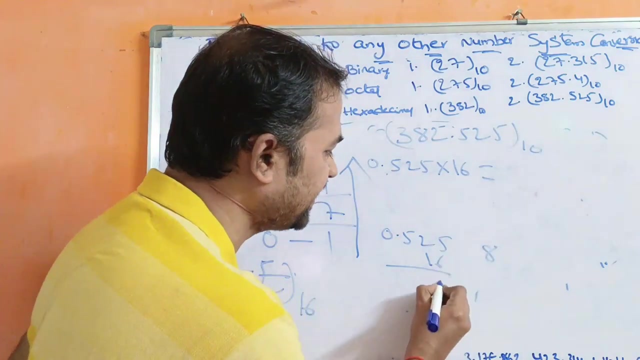 Now we have to calculate For 0.525.. So 0.525 into 16.. Why? Because for fractional part we need to perform the multiplication operation. So 0.525 into 16.. So 16 5s are 80.. 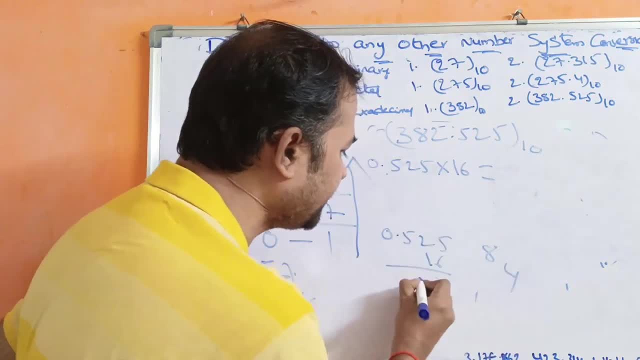 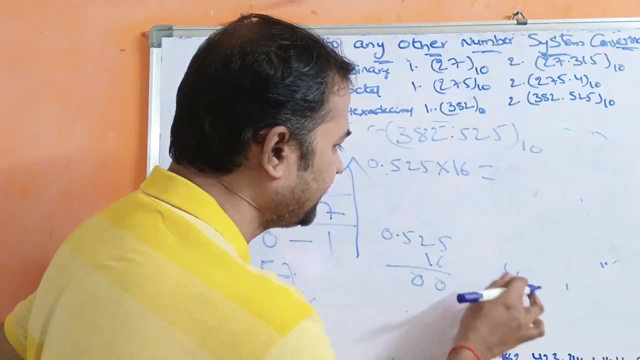 16- 2s are 32.. 32 plus 8 means 40.. 40.. 16- 5s are 80.. 80 plus 4 means 84.. 84. So let us write 84.. So let us write 84 here. 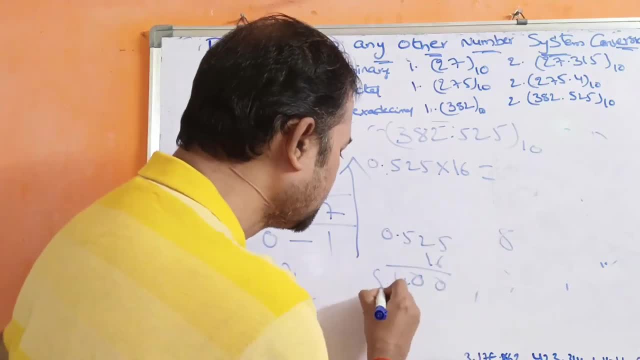 4 here, 4 here, 4 here, 5 here, 5 here, 4 here, 6 here, 16, 0s are 0. So 8.. After one position, we need to write the dot. 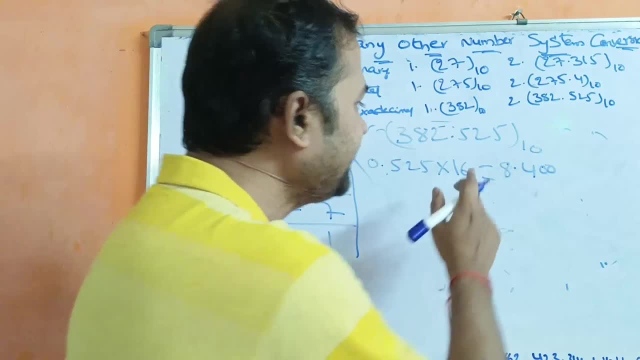 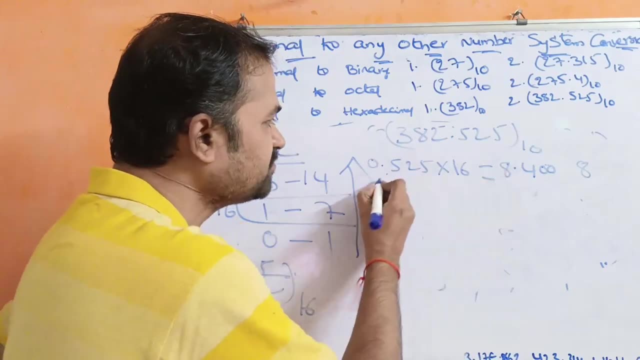 So what is the solution? 8.400.. In 8.400, what is the integer part? 8 is the integer part. Let us extract that integer part and write here. So, after extracting integer part, then it will become 0.. 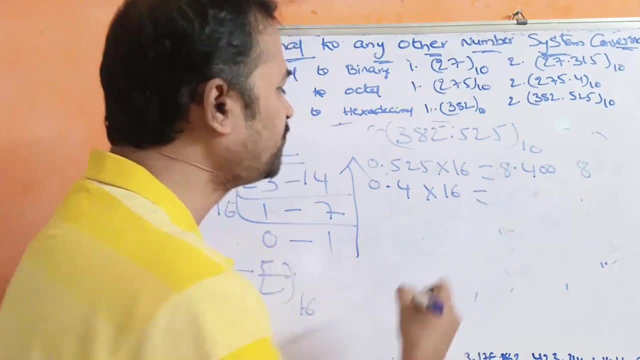 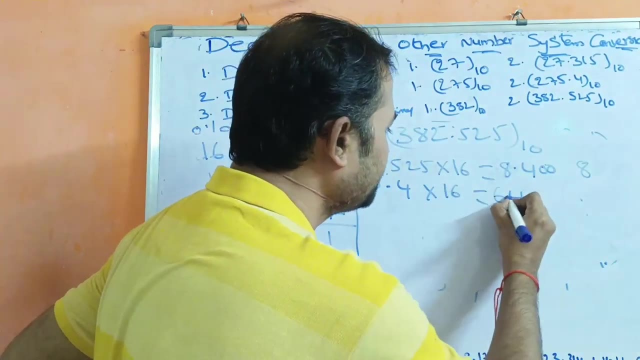 So 0.4 into 16.. So 0.4 into 16 means 16 4s are 64. 64. 64. 64. 64.. After one position, we need to write that dot. 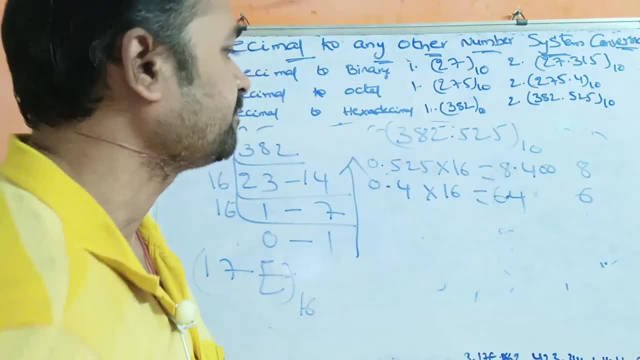 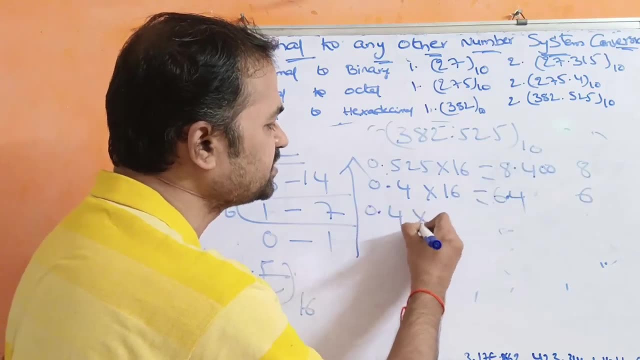 So here, what is the integer part? 6 is the integer part. Okay, Again, it will become what? 0? only After extracting 6, it will become 0.. So 0.4 into 16 means 6.4..